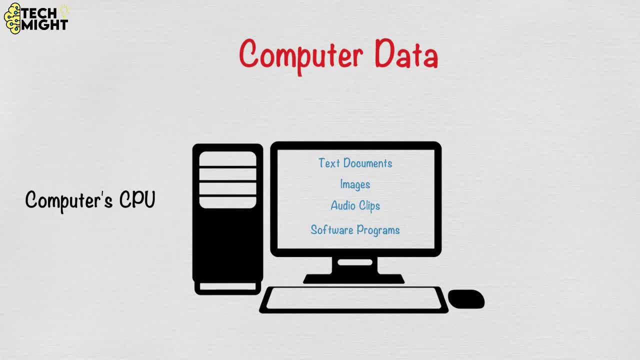 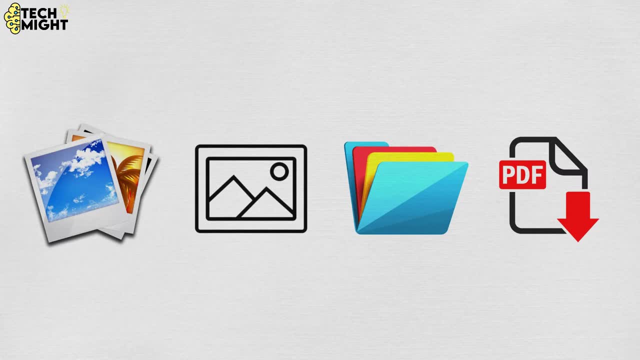 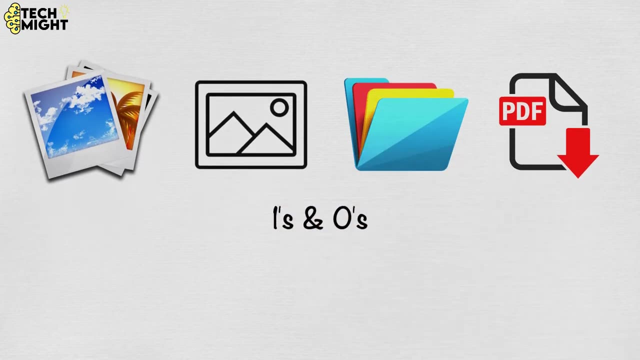 processed by the computer's CPU and is stored in files and folders on the computer's hard disk. A picture, image file, PDF, etc. can also be considered data. At its most rudimentary level, computer data is a bunch of ones and zeros, known as binary data, Because all computer 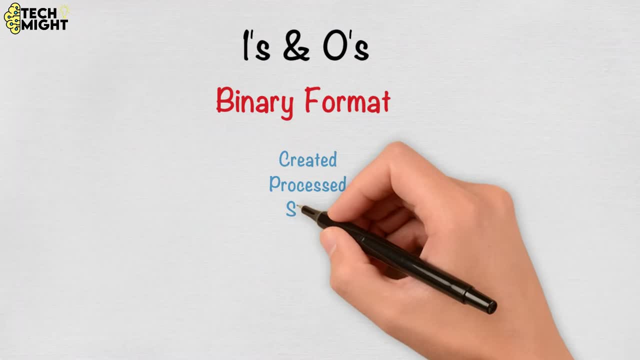 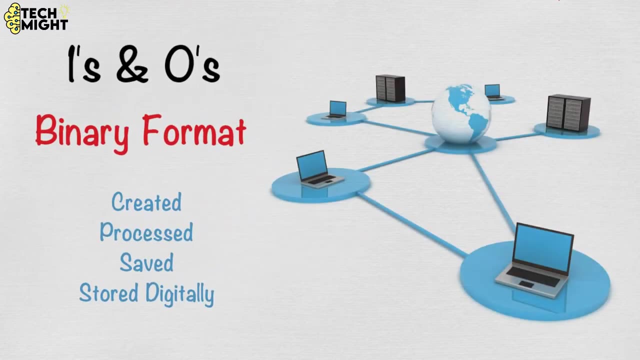 data is in binary format. it can be created, processed, saved and stored digitally. This allows data to be transferred from one computer to another using a network connection or various media devices. It also does not deteriorate over time or lose quality after being used. 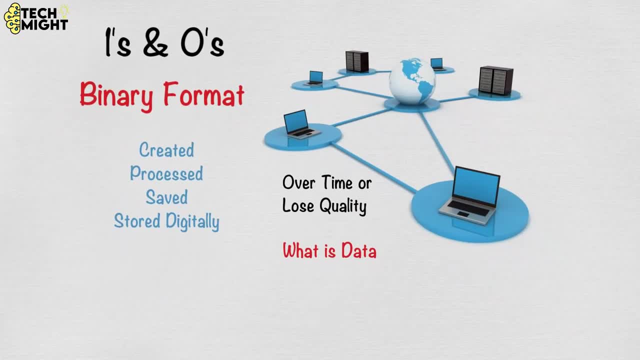 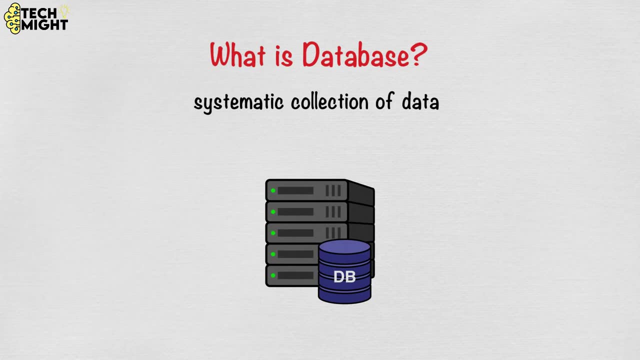 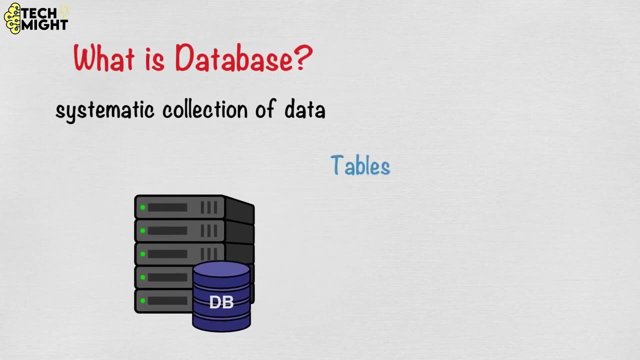 multiple times. So now you know that what is data. Now we will move on to what is database. A database is a systematic collection of data. They support electronic storage and manipulate data. Databases make data management easy. You can organize data into tables, rows, columns. 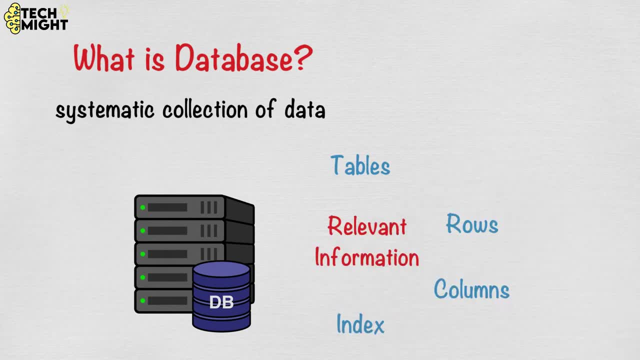 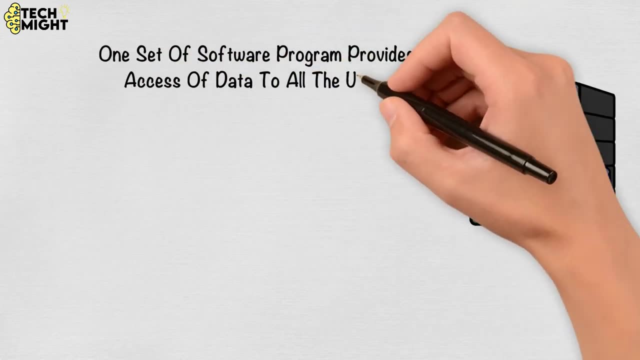 and index it to make it easier to find relevant information. Database handlers create a database in such a way that only one set of software program provides access of data to all the users. The main purpose of the database is to operate a large amount of information by storing 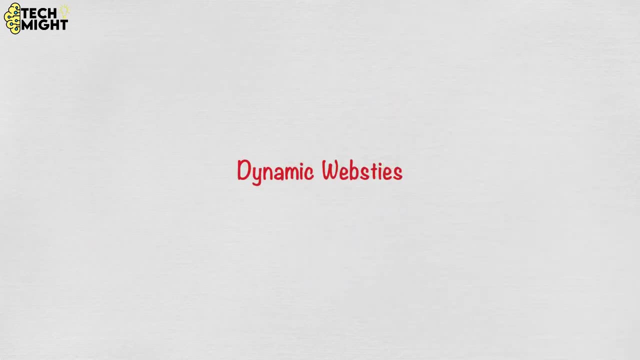 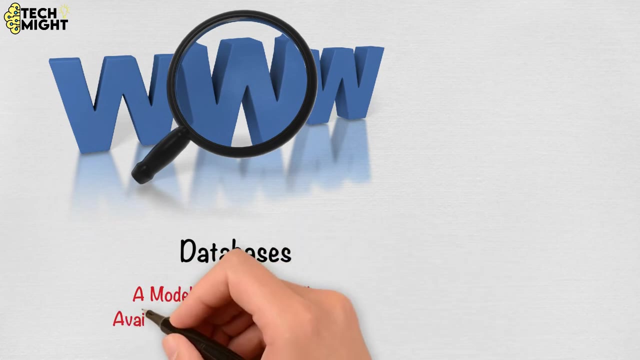 retrieving and managing data. There are many dynamic websites on the world wide web nowadays, For example, a model that checks the availability of rooms in a hotel. It is an example of a dynamic website that uses a database. Let us discuss another database example: An online telephone. 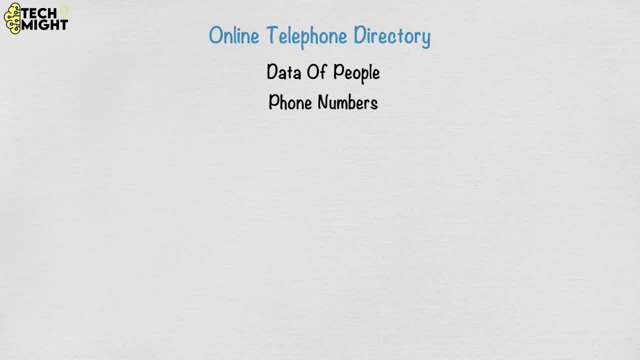 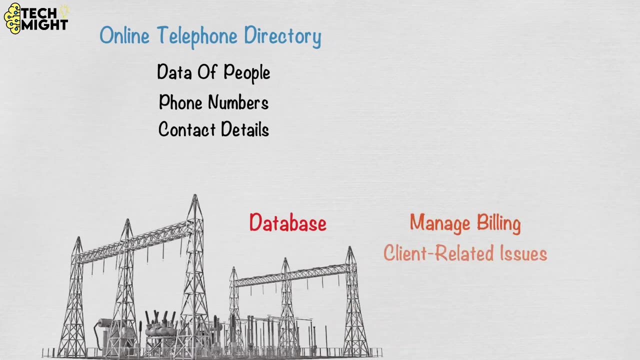 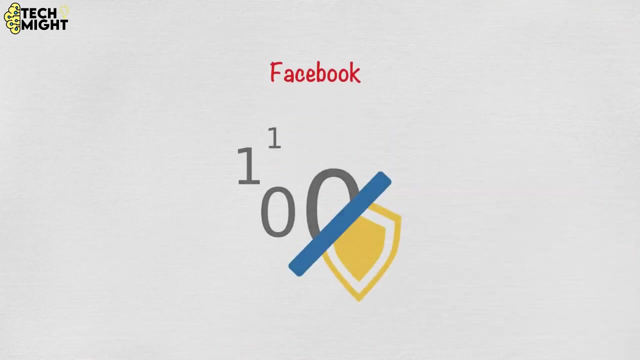 directory uses a database to store data of people, phone numbers and other contact details. Your electricity service provider uses a database to manage billing, client-related issues, handle fault data, etc. It needs to store, manipulate and present data related to members, their friends' member activities. 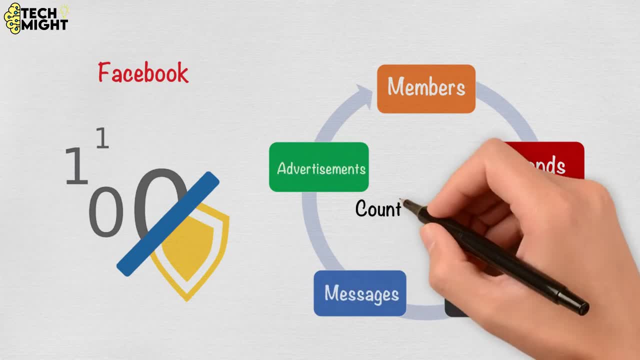 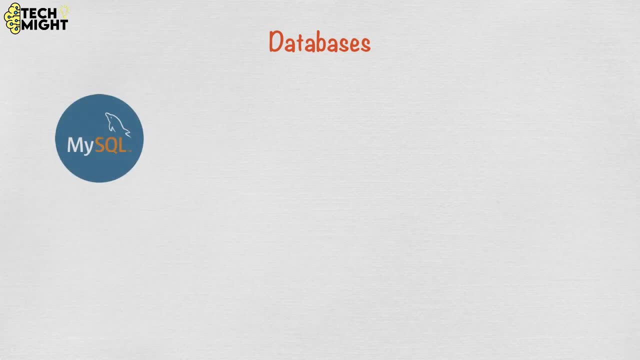 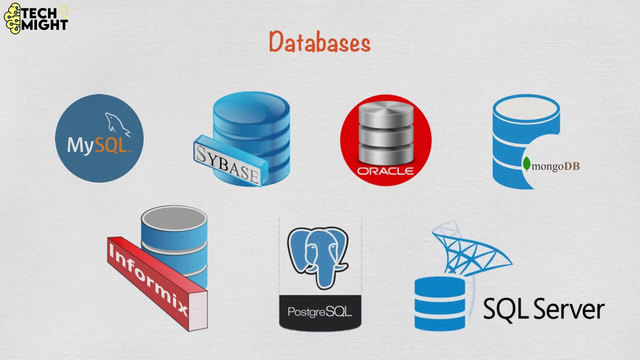 messages, advertisements and a lot more. We can provide a countless number of examples for the usage of databases. There are many databases available, like MySQL, Sybase, Oracle, MongoDB, Informix, PostgreSQL, SQL Server, etc. Modern databases are managed by the database management.